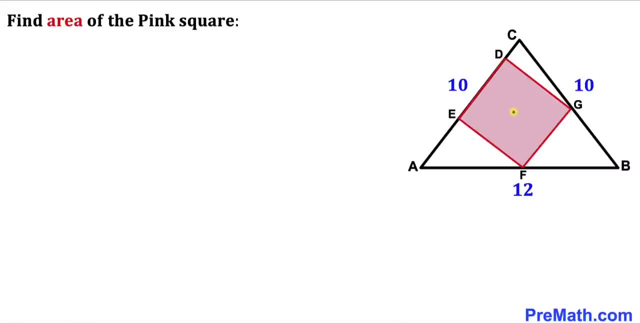 Welcome to PreMath. In this video we have got this pink square DEFG fully inscribed in an isosceles triangle, ABC, as you can see in this diagram, such that this side length, AC is 10 units and this other side, length, BC, is 10 units as well, and, moreover, this side length AB is 12. 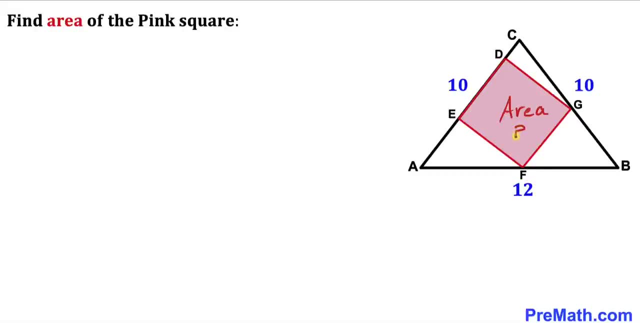 and now our task is to calculate the area of this pink square, DEFG. Please don't forget to give a thumbs up and subscribe. Please keep in mind that this figure may not be 100% true to the scale. Let's go ahead and get started, and here's our very first step. Let's focus on this. 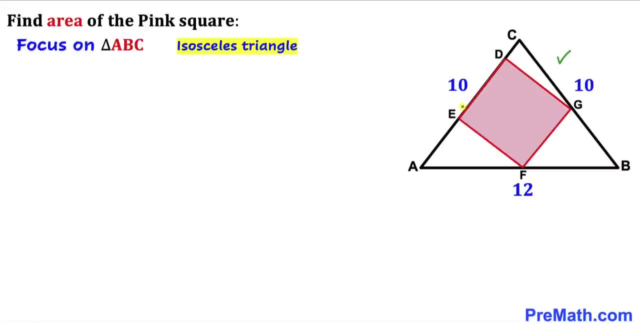 bigger triangle, ABC, and we can see that this is an isosceles triangle. since these two side lengths have a big triangle, Let's go ahead and get started. So therefore, we conclude that this angle is going to be equal to this angle, If I call this angle. 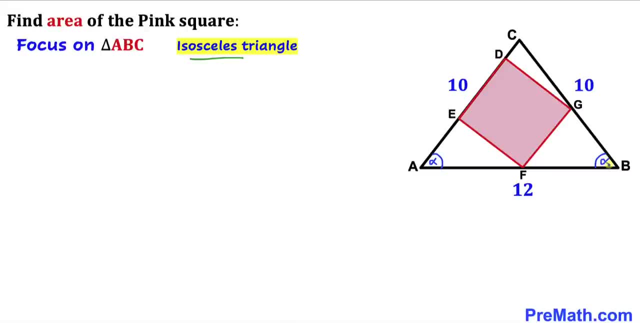 alpha, then this angle has got to be alpha as well. and here's our next step. Let's focus on this pink square. We can see that this side length ED is parallel to this side length FG, So that means this angle has got to be congruent to this angle. So let's go ahead and get started. 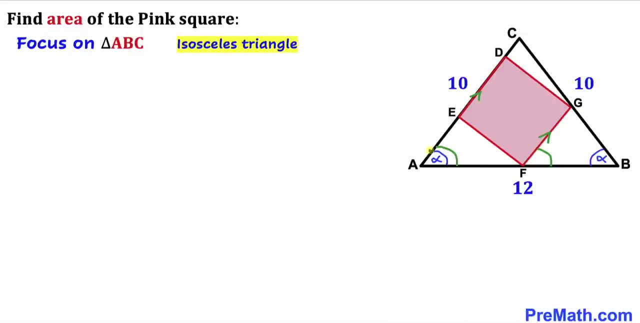 So, therefore, we conclude that this triangle FGB is an isosceles triangle as well, since this angle equals to this angle. So, therefore, we conclude that these two triangles, this triangle FGB and this big triangle ABC, are going to be equal to this angle. So let's go ahead and get started. 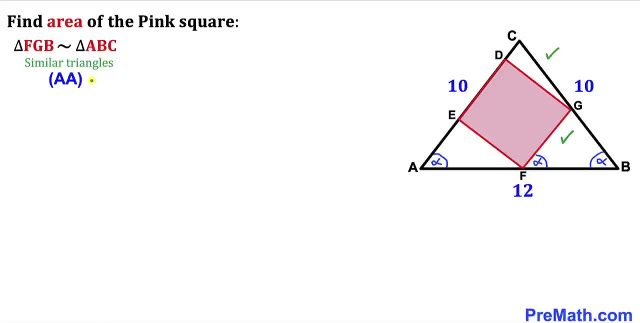 So therefore, we conclude that this angle is going to be equal to this angle. So that means their side lengths are going to have the same proportion. If this side length is 10, then this side length has got to be 10 times some constant a. Likewise, this side is going to be 10 a, and this 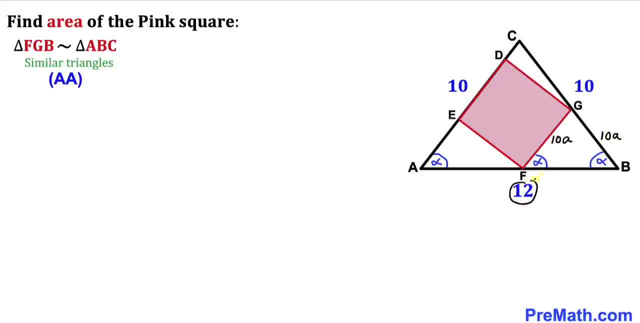 side is going to be, according to this, 12. that is going to give us 12 times 10.. So that means that the side length is going to be equal to the segment AB. So we conclude that this angle is parallel to this angle. So let's start the second step. We have to work out the state length as well. 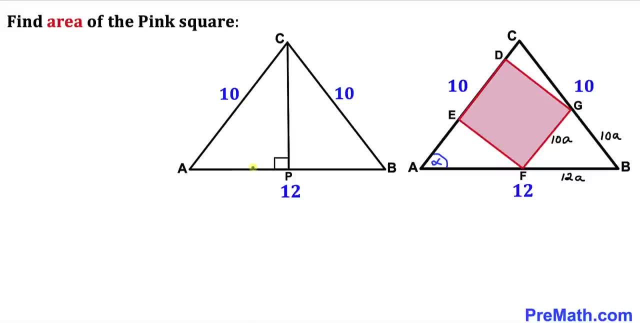 So if we want to go ahead and get the side length of the right side, so we have to calculate the line length and we will need to calculate the section length as well. So let's go ahead and let's start with this section length. So let's say that this is the section length AB, So we need to. 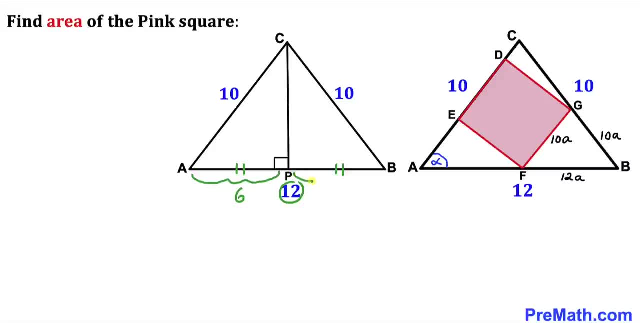 of this 12, that is going to be 6 and this is going to be 6 as well. and now let's focus on this right triangle, APC, whose side lengths are 6 and 10. we are going to calculate this side length, PC. and now let's recall the 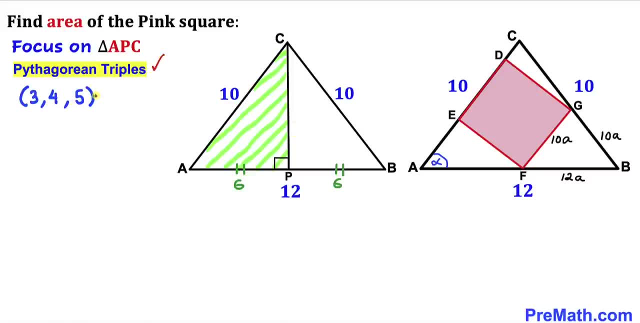 Pythagorean triplets: 3, 4, 5. if we multiply these triplets by 2 across the board, then our new pythagorean triplets are going to become: 3 times 2 is going to give us 6, 4 times 2 is going to give us 8, and 5 times 2 is going to. 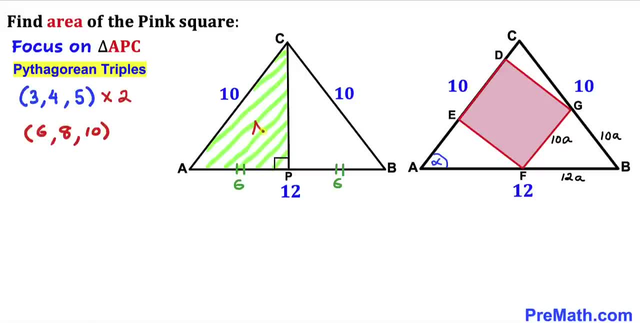 give us 10, therefore, in hour, this right triangular APC. if this side length is 6- this is 10- then this side length CP is going to be 8. so, therefore, our this unknown side length CP turns out to be 8, then we multiply and now let's talk about CP. the unknown side length is going to get. to be 8 and so the stay honesty of this particular side length is to be 406. you cannot get impossible side length CP because it is 8 s the manipulative side length. parallel difference between side length and CP, which 6 and 9 of these necessary. 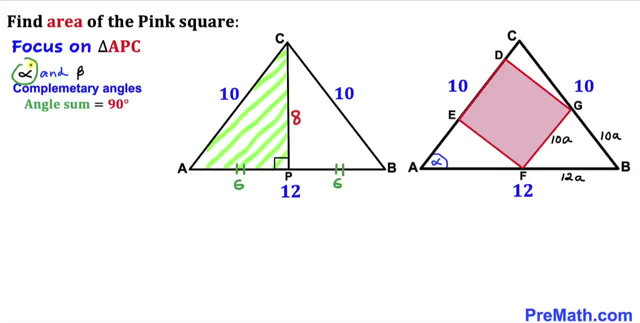 units. and here's our next step. let's assume that alpha and beta are our two complementary angles, in other words, some of these two angles, alpha plus beta, is going to be equal to 90 degrees. let's assume that this angle is alpha, if this is our 90 degree angle. 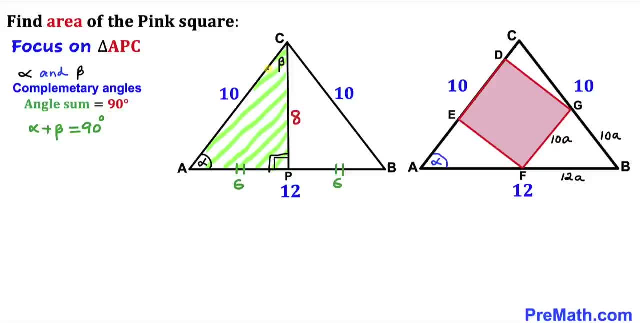 then this angle has got to be our angle beta. and here's our next step. let's focus on this right triangle, aef, and we know our this angle is alpha. this is our 90 degree angle. so therefore, this angle has got to be our angle beta. so therefore, we conclude that these are two right. 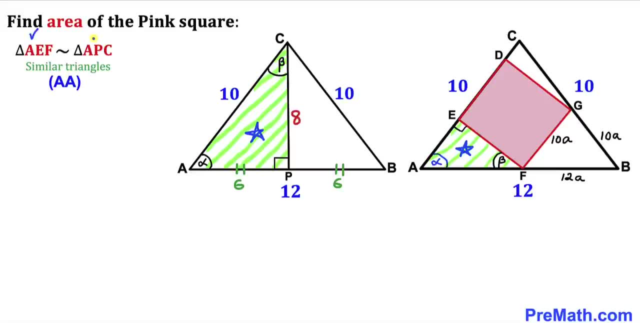 triangles aef and this triangle apc are similar triangles according to angle angle similarity theorem, so therefore their side lengths have a same proportion. if we look at this 10, then this side length af is going to become 10 times some constant b. if this side length is 6, then this side length a is going to become 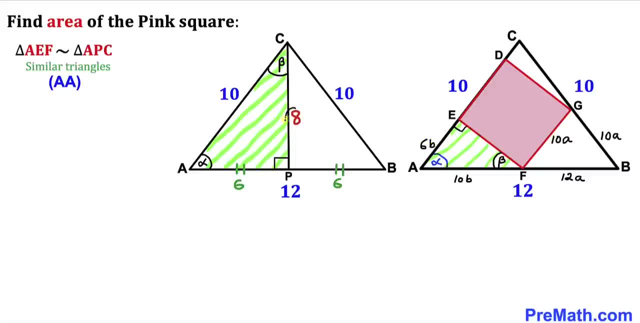 6 times b and finally, for this side 8. this length is going to become 8 times b. and here's our next step. let's focus on this pink square defg. so that means all these side lengths are going to be equal. if i call this side length x, then this side length is going to be x, x and x. 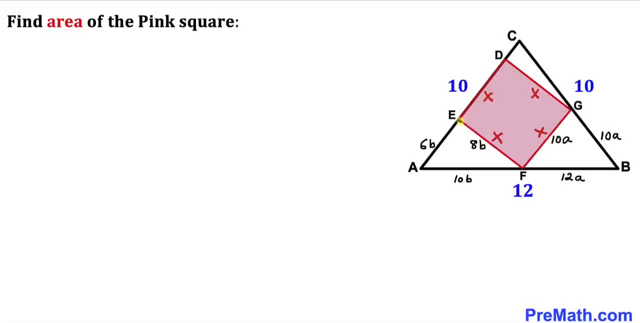 across the board. and now let's make an observation. look at this side length. ef. this is equal to 8 b. therefore we can equate them. therefore, we can write: 8 times b equals to x. let's divide both sides by 8. so therefore our b value is going to become x divided by 8. now let's focus on this side length. 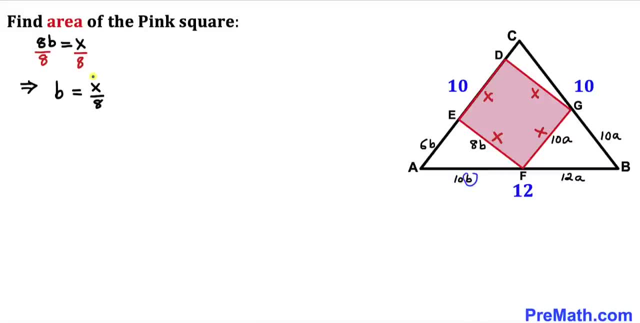 10b and we know our b value is x divided by 8, so therefore i'm going to replace this b by x divided by 8. so therefore this could be written as 10 times x divided by 8 and if we simplify, that could be written as 5 x divided by 4. so therefore this 10 b could be replaced by 5 x divided by 4. 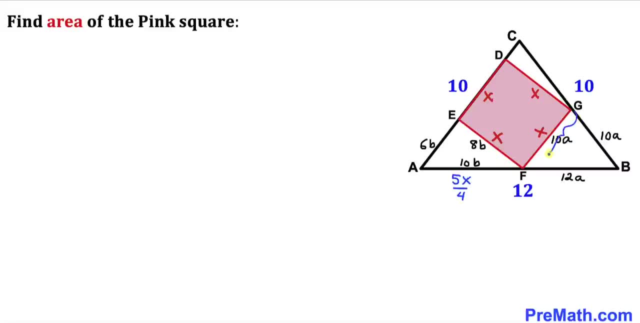 and here's our next step. let's focus on this side: length, fg. that is equal to 10 times a and that is also equal to x, so i can equate them as well. so therefore, i can write: 10 times a equals to x. let's divide both sides by 10 to isolate a. so therefore, our a value. 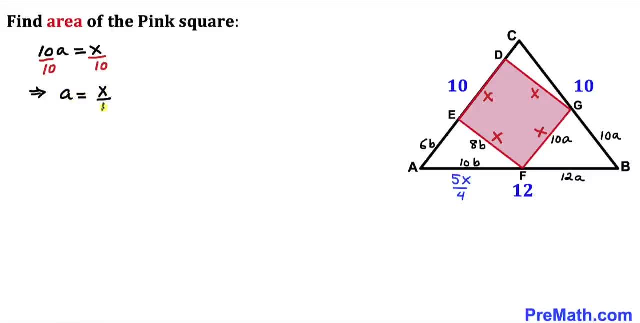 turns out to be x divided by 10. and now let's focus on this side. length 12, a and our this a value is x divided by 10, so i'm going to replace this a by x divided by 10 over here. so therefore, i can write 12 times x divided by 10, and if we simplify this thing, that is going to give us: 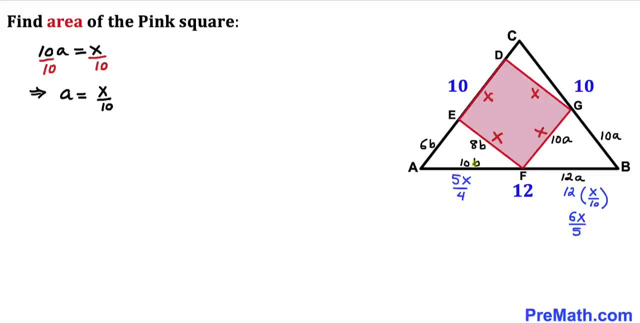 6 x divided by 5. so therefore, i'm going to replace this 12 a by 6 x divided by 5. and now let's make an observation. we can see that this whole side length a b is going to be equal to this: 5 x divided by 4. 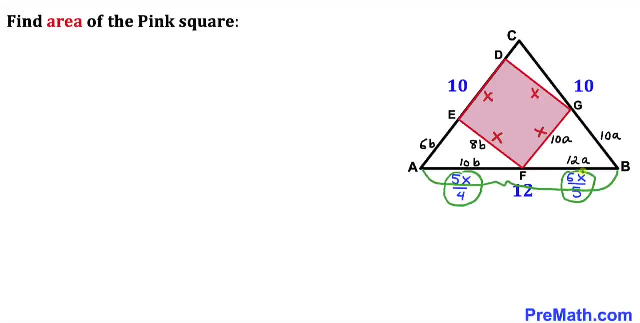 plus 6 x divided by 5, and this side length, a, b, is also equal to 12, so i can equate them: equals to 12. so therefore i can write: 5 x divided by 4 plus 6 x divided by 5 equals to 12. and now we can see if we look at the denominator 4 and 5. 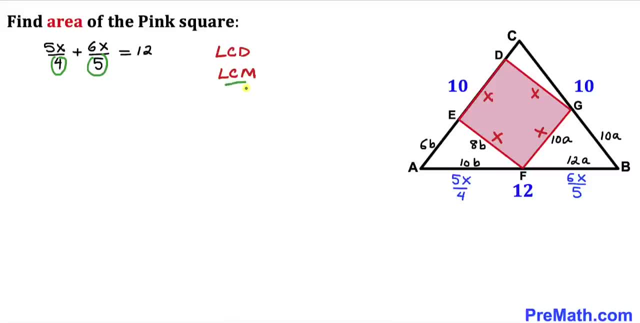 our least common denominator, or sometime we call it least common multiple, is going to be equal to 20.. so, therefore, i'm going to multiply both of these terms by 20 and, on this side, 20 as well, across the board, and now we can see that 4 goes into 25 times, 5 goes into 20. 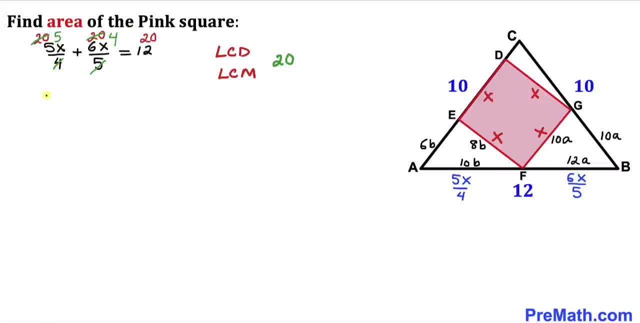 4 times. so therefore, 5 times 5 x is going to give us 25 x, plus 4 times 6 is going to give us 24 x, equal to 240 on the right hand side. so therefore let's combine the like term that's going to give us.